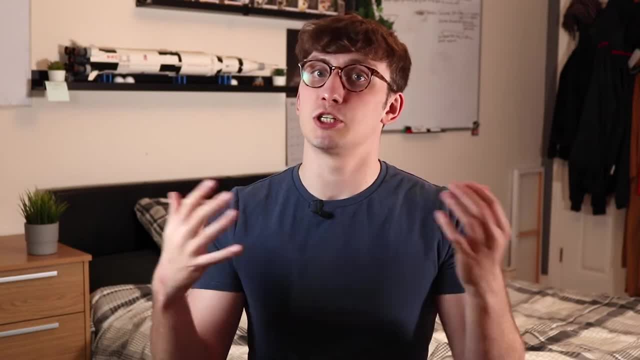 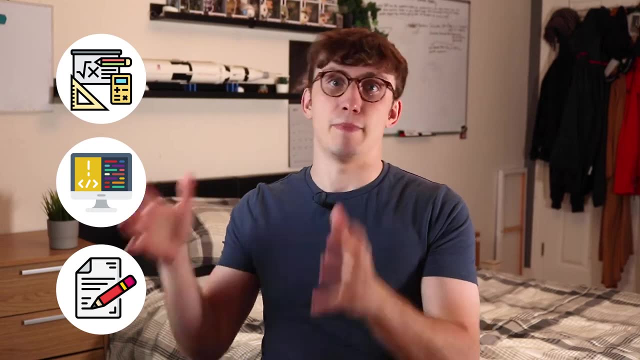 things that I wish I knew before I started, And so, in today's video, I'm going to share those things with you, And this video is going to be split broadly into two parts: First of all, the skills that you need, and then the mindsets and attitudes you need before going into study. 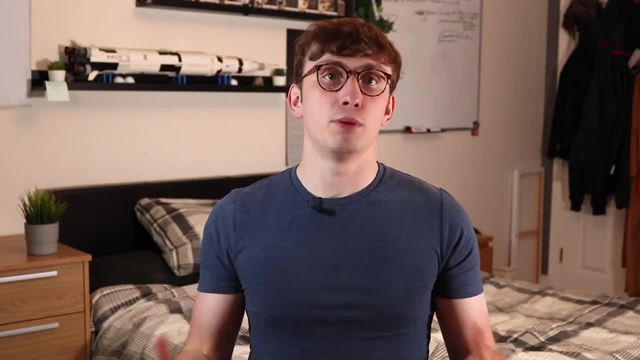 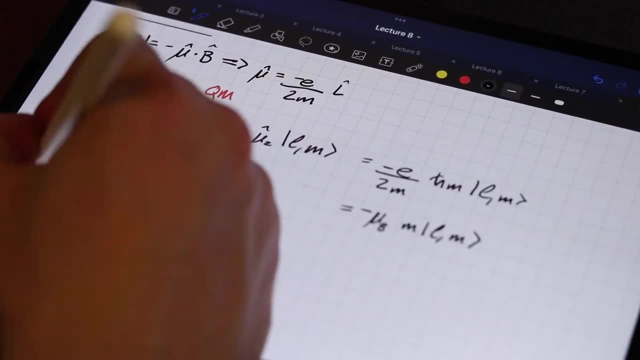 So let's begin with the skills. As you might guess, one of the most important skills when it comes to learning physics is maths. Maths is the language of physics, It's the language of science And, no matter how much you try, there's no getting around the fact that maths is a key. 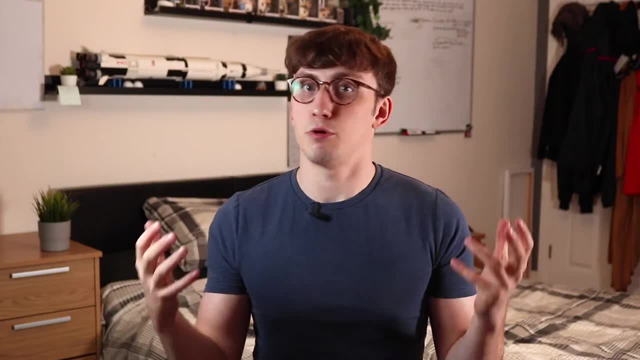 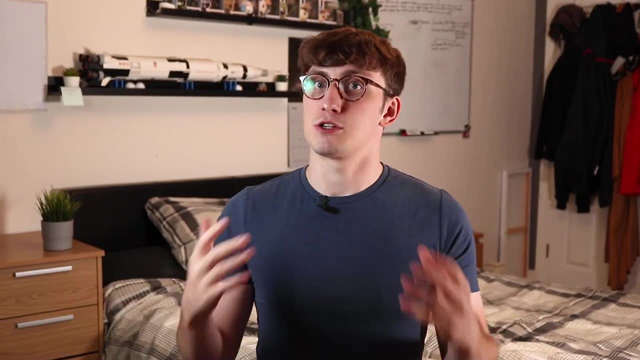 component of a physics degree. Now, the fact that you study in physics probably indicates that you have some proficiency with maths already, which is great, And even if you didn't get the grades you wanted in maths, that's not a problem. In fact, maths was my weakest subject at A-levels. 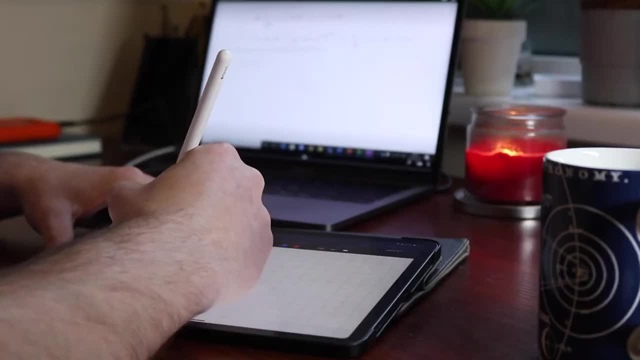 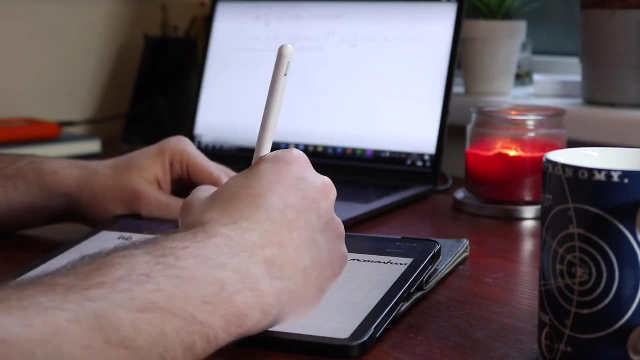 and I still went on to study physics and get a first at the end. Now, when it comes to practicing maths, there are a few different methods that you can use, depending on the style that you like to learn and how much time you have. So the first method, and perhaps the most basic method, is the 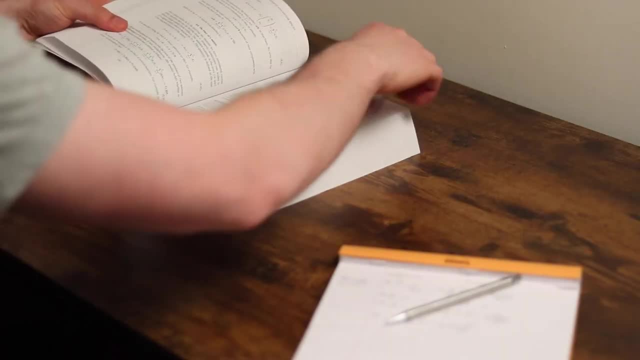 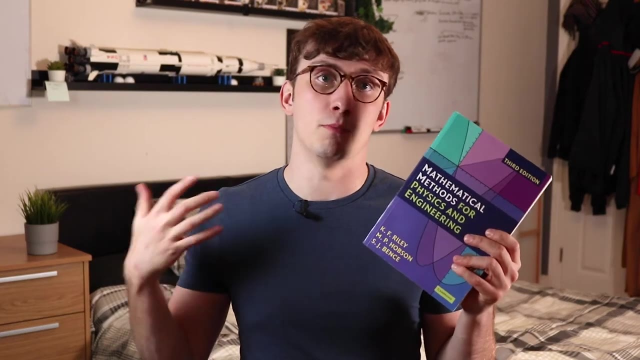 classic textbook. This is just getting a maths textbook and going through the chapters that you find most difficult or that you need a refresher on, or the chapters that are going to come up in your modules during university. So this is the textbook I would recommend for maths. 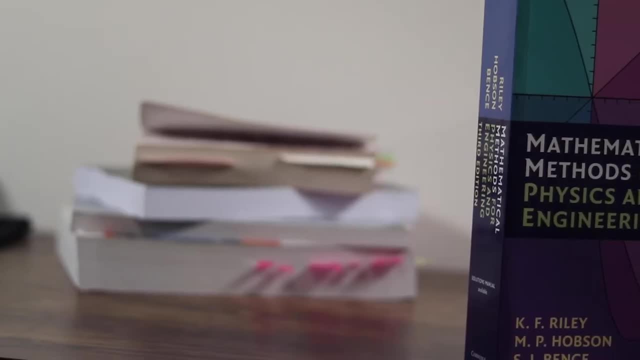 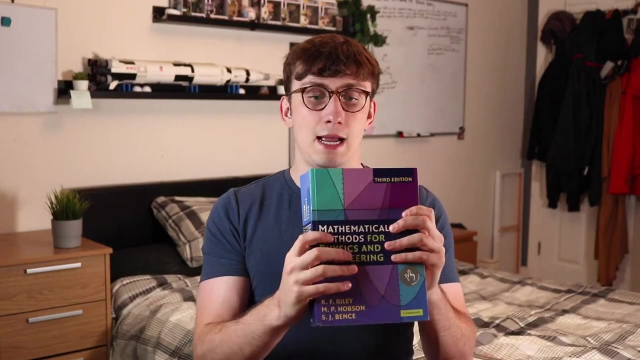 It's called Mathematical Methods for Physics and Engineering, And if you're a physics student or an engineering student, this is pretty much the standard textbook that you're going to use at university, no matter where you go, And that's because basically all of the maths that you're 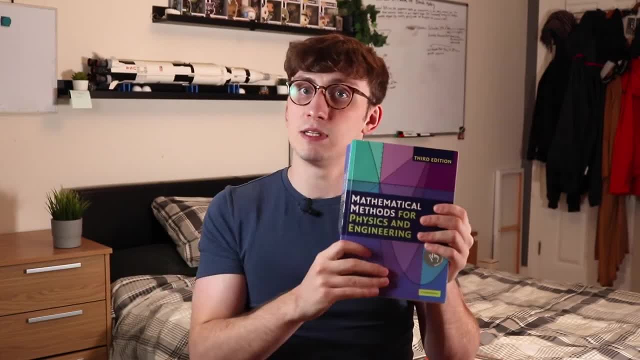 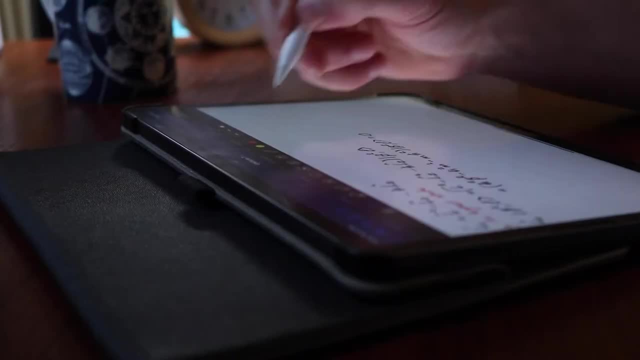 going to need throughout your degree is going to be in this textbook, And the good thing about these types of textbooks is, at the back of each chapter, there is a section of practice problems, which is the only way you're going to improve at maths is practicing problems, And the reason I 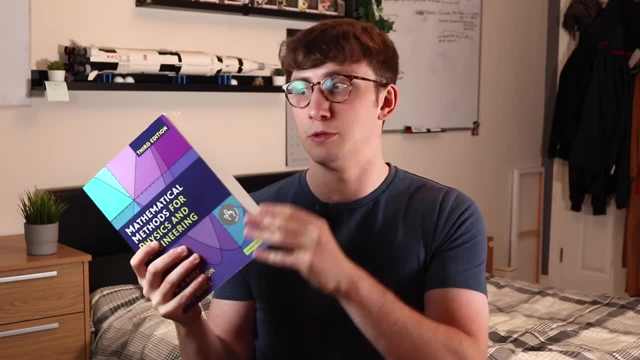 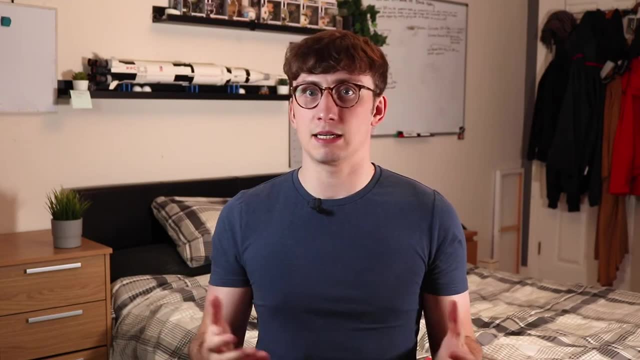 like the textbook method is because if you do struggle with a certain problem, you're going to literally go back a few pages and there's the whole explanation there. Now, if you know there's a specific part of maths that you want to practice, but you don't want to go through the textbooks and 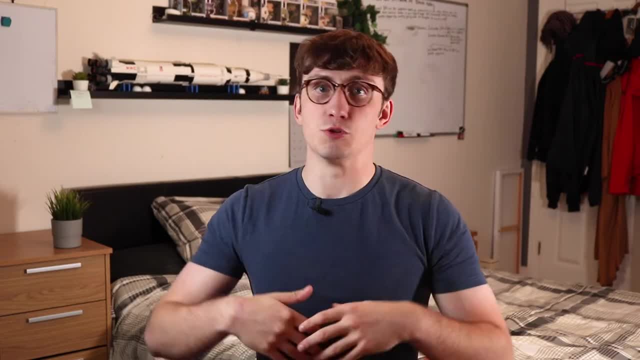 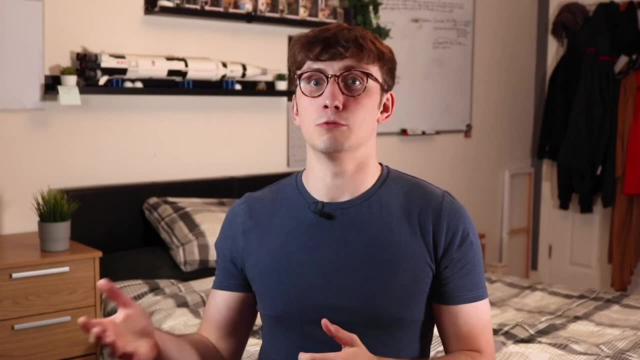 you don't want to watch lectures, then another method you could use is using other online resources. So there's plenty of resources online that I'd recommend. You could watch YouTube channels like 3Blue1Brown, which give really great maths explanation videos, Or you could use 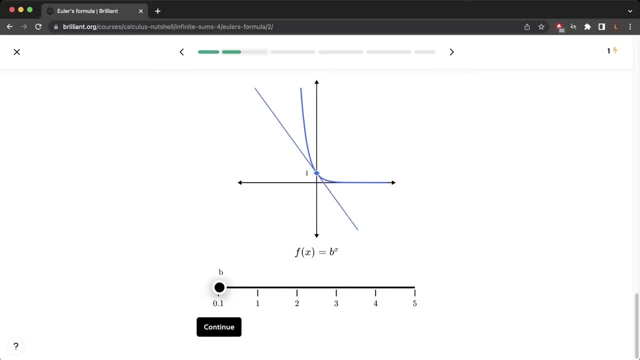 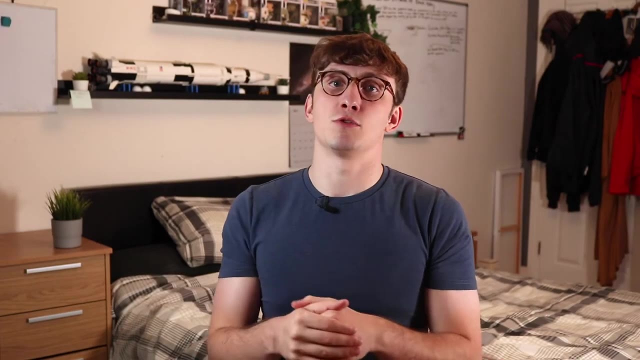 online course websites like Brilliantorg, which give interactive courses on maths which you can sort of practice along while having the explanation given to you, which is a great method, And actually there's a link in the description which you could sign up for Brilliant and get a free trial. Or you could use a resource like Khan Academy, which is 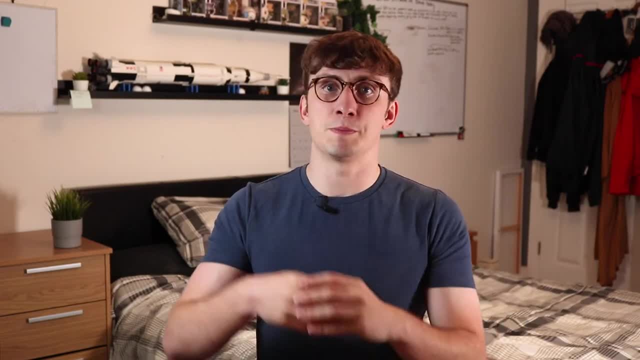 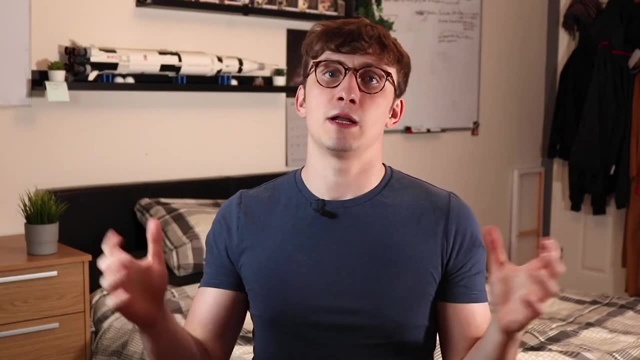 similar to Brilliant in that it's got a lot of practice problems, but also similar to 3Blue1Brown in that it's got explanation videos as well. So, depending on how you like to learn, there's all of these resources that you can use to improve your maths. 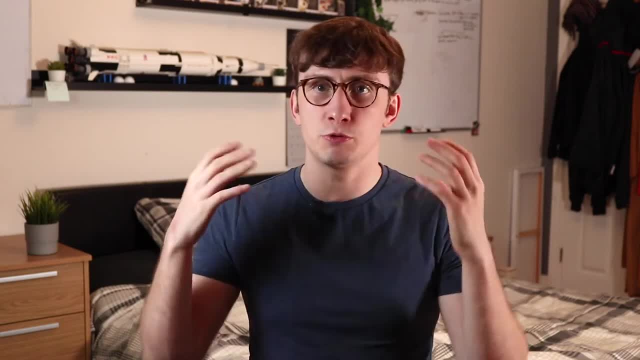 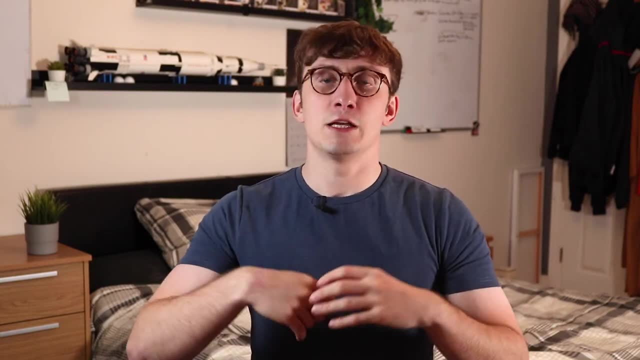 And one thing I would say is: don't focus on it too much. You know you don't need to be an expert in maths. before starting a physics degree, You'll have introductory courses on mathematics, so you don't have to be an absolute expert. The second skill that is absolutely essential when it comes: 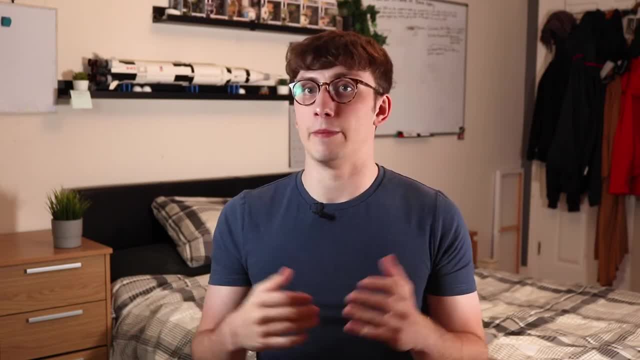 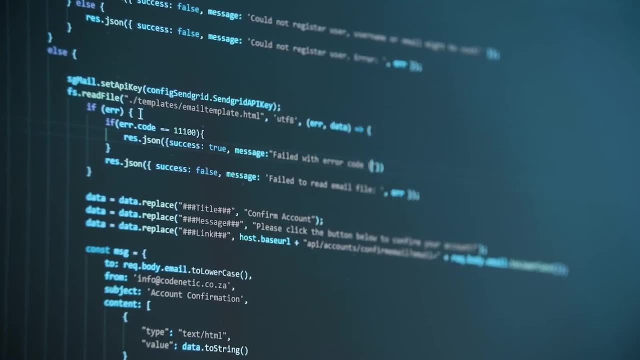 to a physics, and especially astrophysics, degree is programming. Now, I knew that I was going to do some programming during the degree and I knew that I would take modules on programming which would teach me how to code, But I wasn't aware of just how much coding I would do throughout the degree. 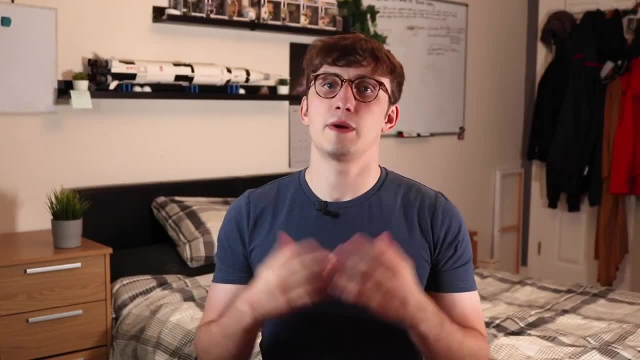 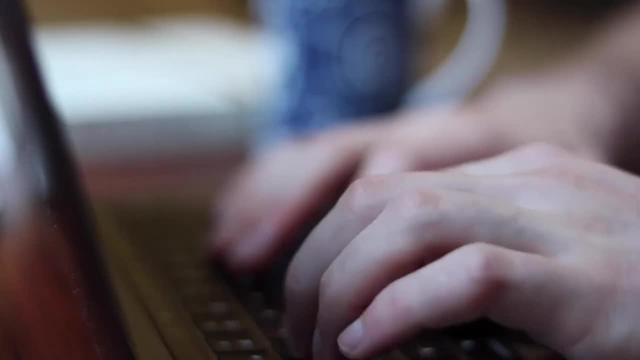 Not just in the coding specific modules. So when it comes to astrophysics, programming is primarily used when it comes to data analysis and visualization. Now, depending on the courses you take at university, you might be taught different programming languages, But the one programming language I would recommend. 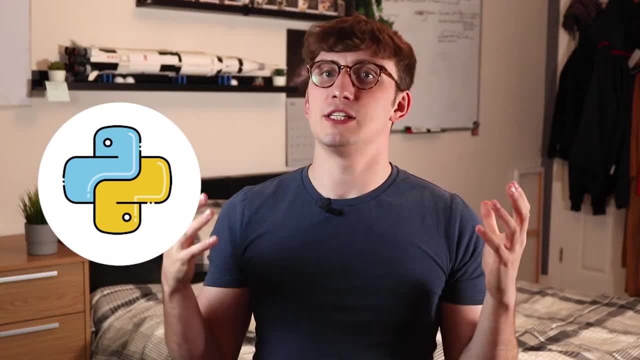 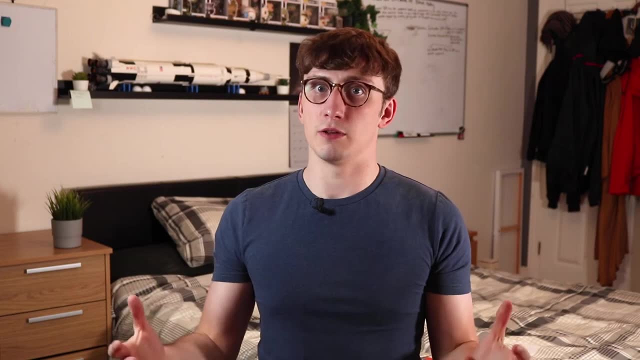 everybody try to learn is Python. Now, Python is universally used throughout physics and astrophysics for its ability to handle large amount of data, which is what's used a lot of the time in physics and astrophysics. Now, the great thing about Python is the fact that it's got a bunch of different packages. 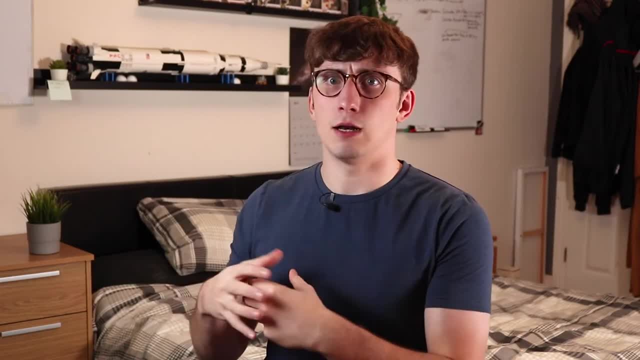 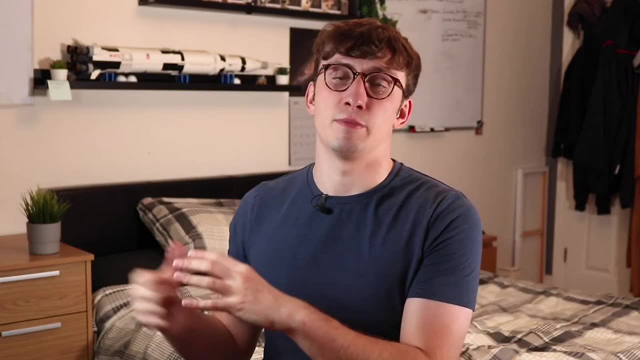 that you can use depending on your requirements. So if you've got a lot of astro analysis to do, you can use the module AstroPy to perform a lot of analysis and visualization of that type of data. Or if you've got some large data set, you can use something like Pandas. 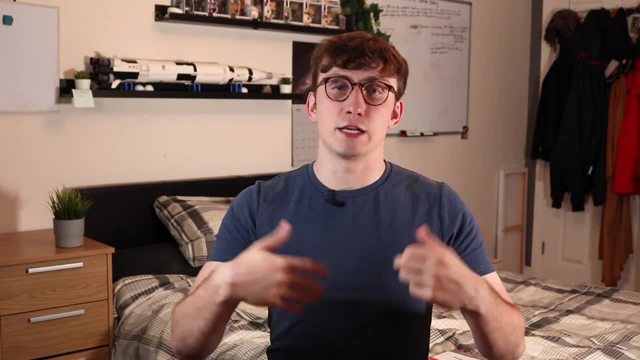 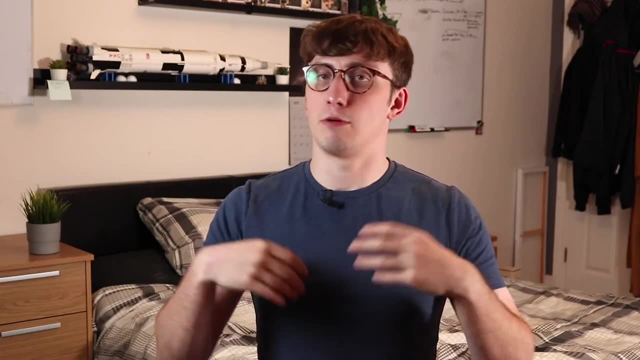 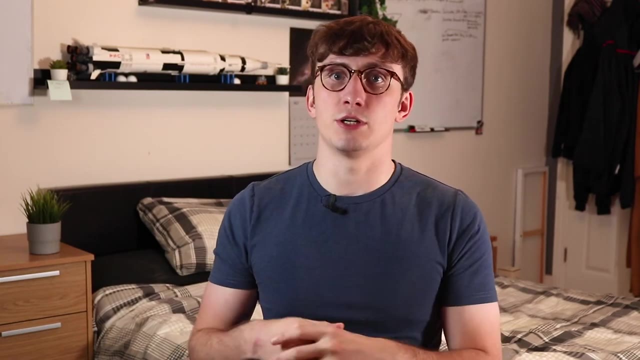 or NumPy to sort and analyze and extract information from that data set and then use something like Matplotlib to plot your data. All of my degree for the research side of the degree in the research module, So through first year, second year and third year, all of the little research and programming modules. 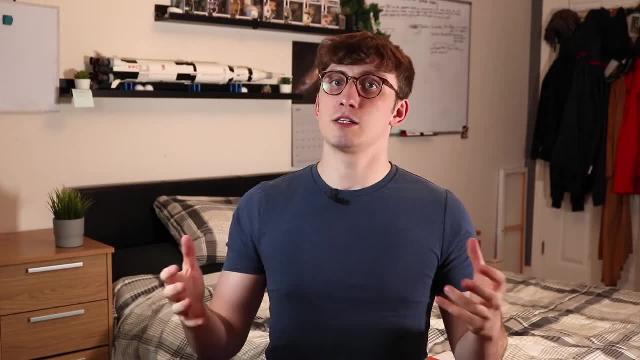 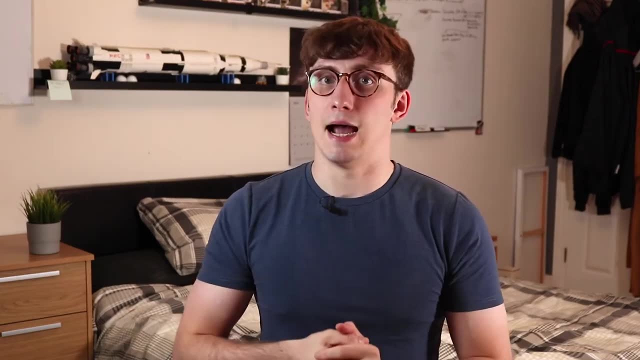 I had. I basically used Python exclusively. So if you are going to study physics, I would highly recommend that you learn Python. It's, like I said, pretty much universally used throughout all of physics and astrophysics And it's one of the easiest programming languages. 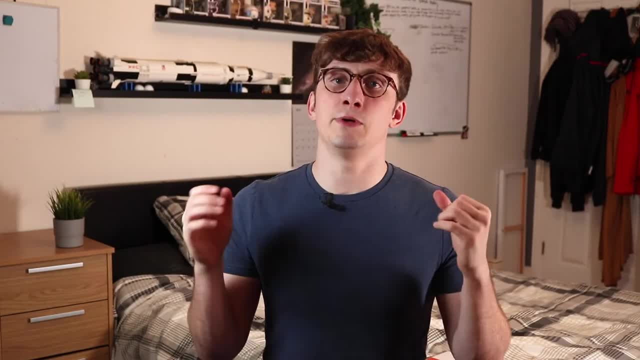 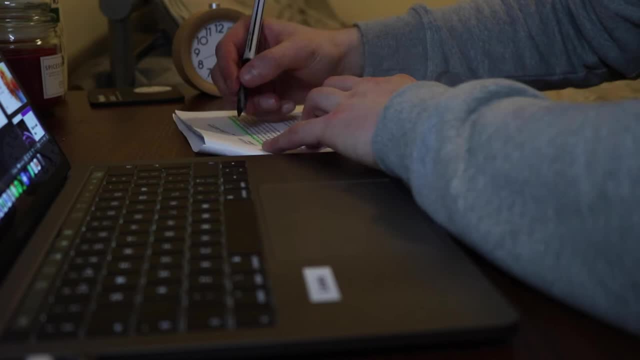 to pick up as well, which is always great. And the final skill that I think is absolutely essential to a physics student is scientific- Okay, Scientific- writing. This is something, again, that you don't necessarily immediately think of when it comes to physics, but being able to write in a scientific style and express 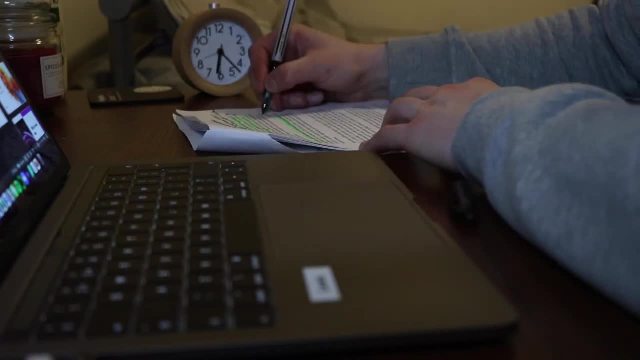 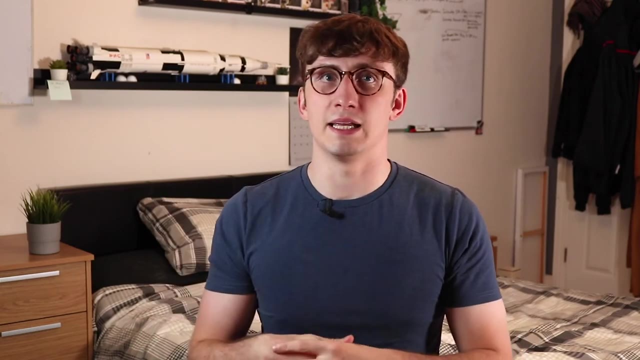 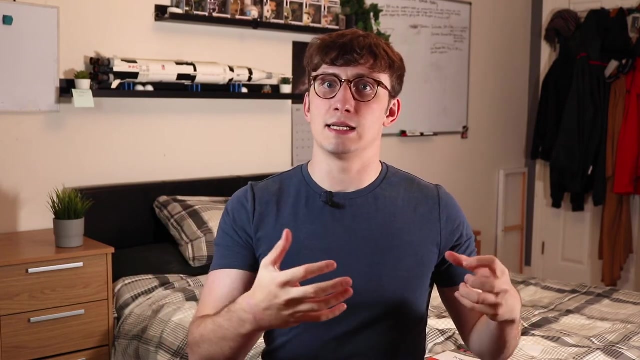 your ideas and your results in a way that anybody can understand is an extremely important skill. Now, this doesn't mean writing in an extravagant and flamboyant way. What it means is simply expressing complicated thoughts and complicated ideas in a simple to understand and easily accessible way. 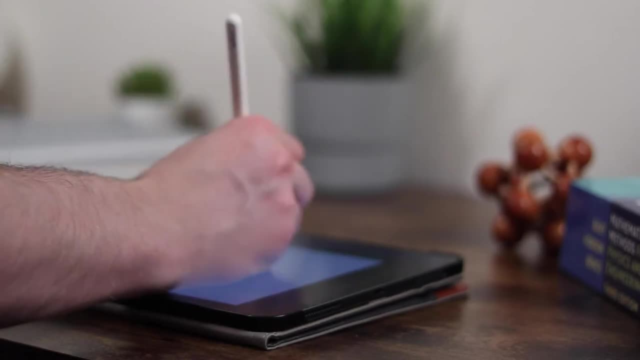 One of the best pieces of paper that I've ever written is the one that I've ever written. One of the best pieces of paper that I've ever written is the one that I've ever written, and the most effective advice I had during first year was to not write complex sentences. 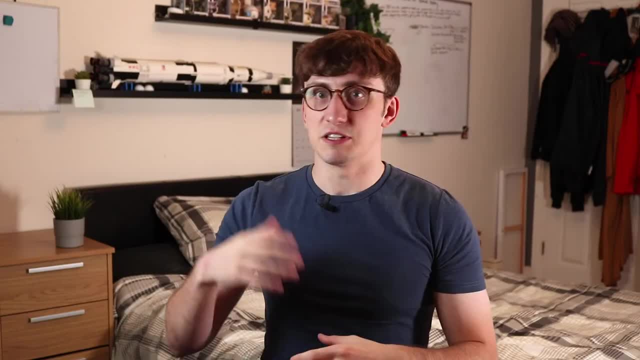 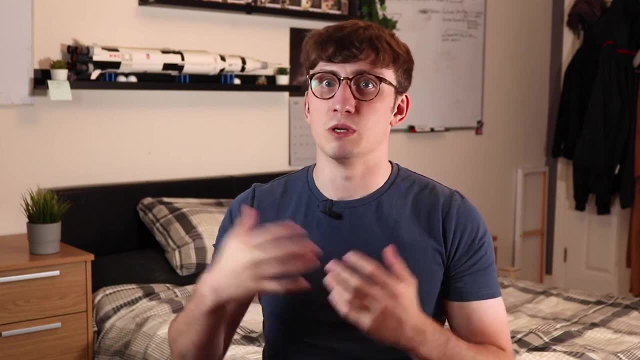 to try and sound academic and try and sound smart If a simple sentence will do, use it, And I've applied that sort of idea throughout all of my writing and always received great grades because of it. So you might be wondering where in astrophysics you're going to be needing. 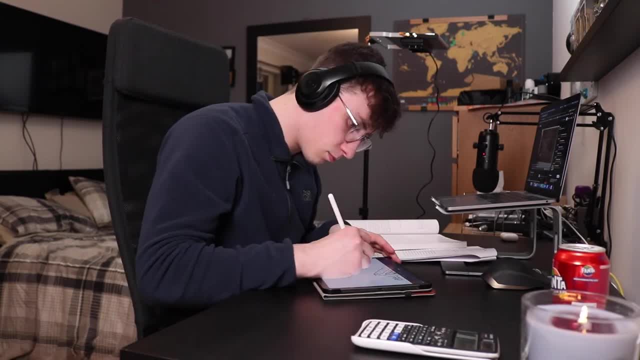 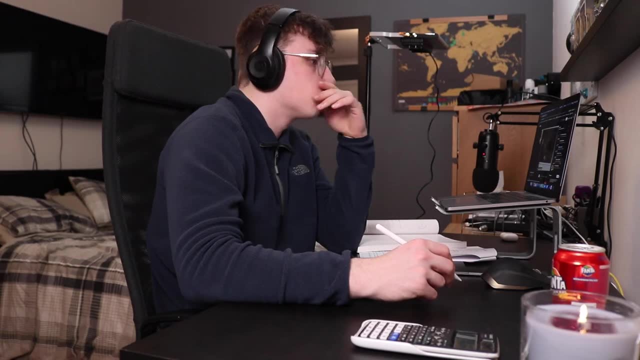 to write so much, And it's actually far more common than you may think. So for reference, during my degree I did about three or four little research projects which sort of built on the foundation of scientific writing that I had, And during these 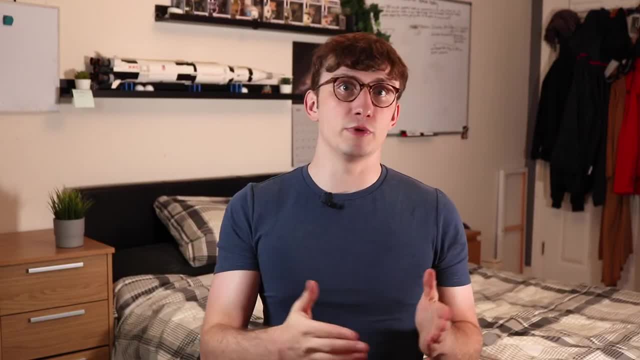 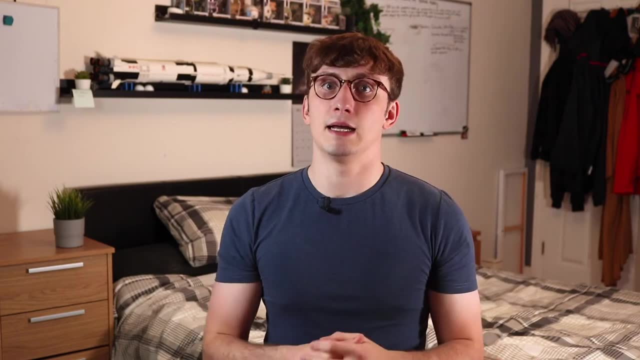 sort of little research projects. we was expected to perform the whole research and explain our methods and our process and our results. So being able to write in an elegant manner is a pretty important skill as well. So I'd say those are the three foundational skills that you're going to 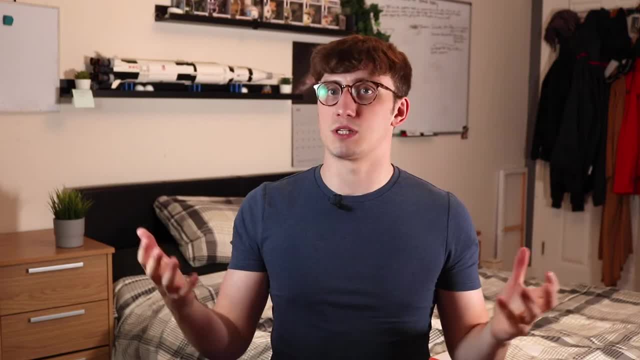 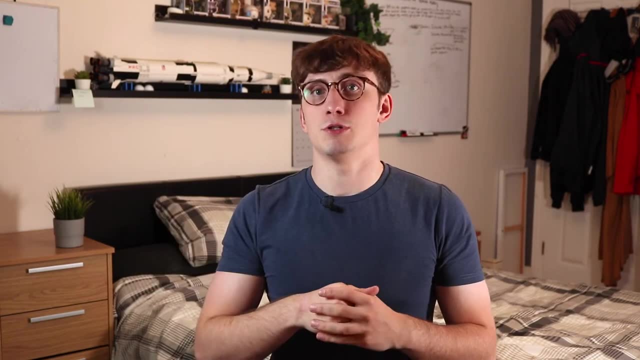 need as a physics and astrophysics student. Obviously, you're going to need more skills than that. You're going to need study skills, exam skills, time management skills and a lot of management skills, And I've actually made a video on how to study for exams, which I 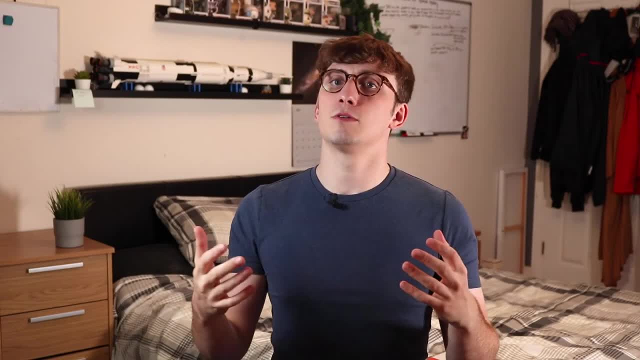 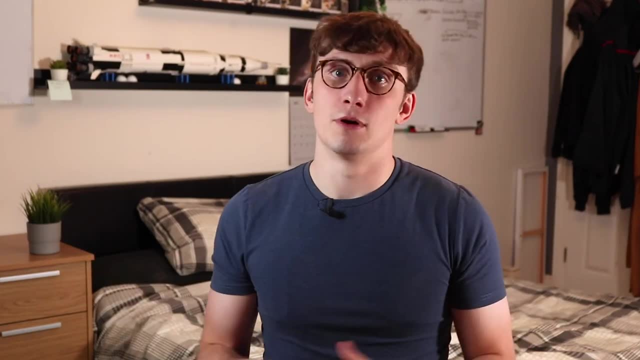 will link up there, But that's not all you're going to need Now. we'll talk a little bit about the mindset and attitudes that we're going to need in order to succeed at physics and astrophysics. First, and probably most importantly, you're going to need to be passionate. 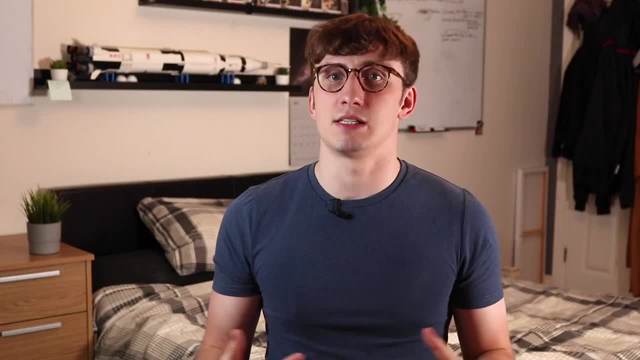 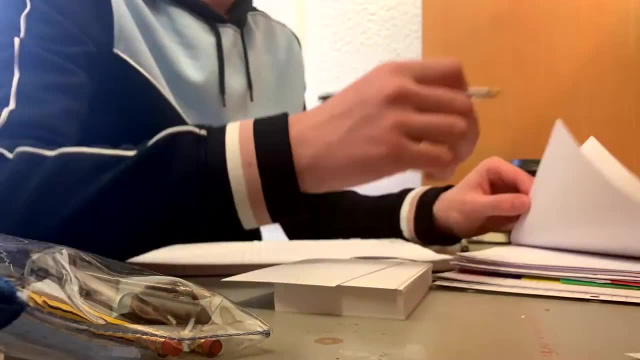 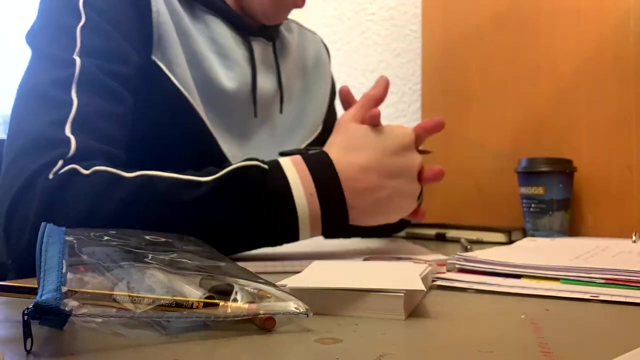 Astrophysics is widely regarded as one of the most complicated and difficult subjects to learn and to study, And with good reason. I mean it combines complex maths with abstract theories in a pretty difficult to understand combination. And if you haven't got that passion, 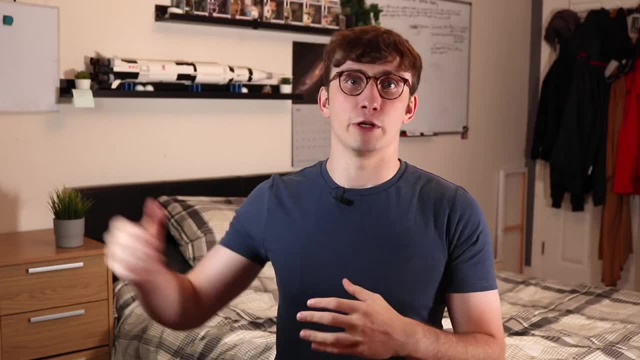 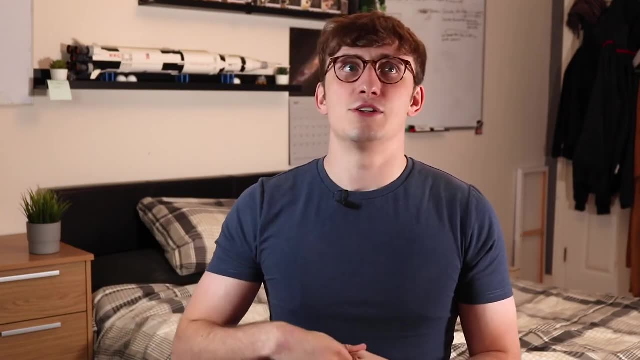 it's going to be pretty difficult for you to see out the three or four years that you're going to study astrophysics. If you're studying astrophysics to sort of prove that you can do the hardest subject, or to sort of show that you can understand these complicated theories, rather than doing it, 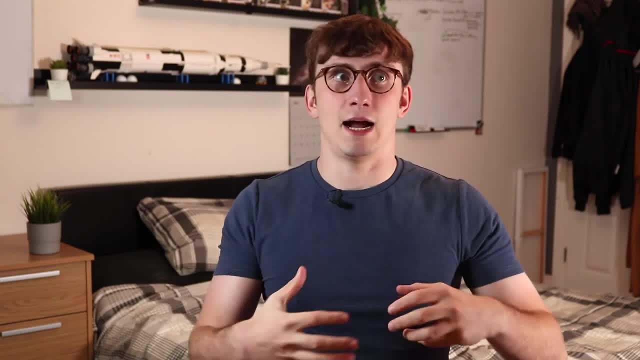 because you want to understand how the universe works and how these unbelievable massive structures in the universe work. So I'm going to show you how to do that And I'm going to show you how to know how the universe works and how these unbelievable massive structures in the universe 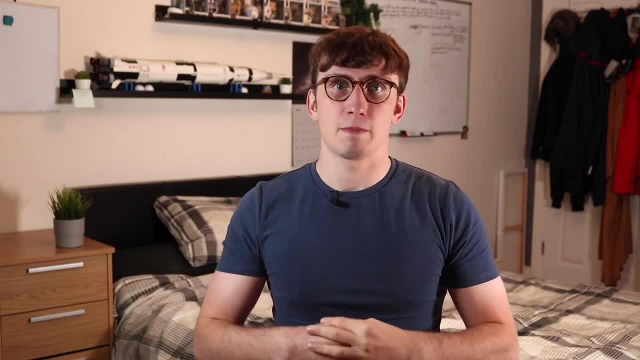 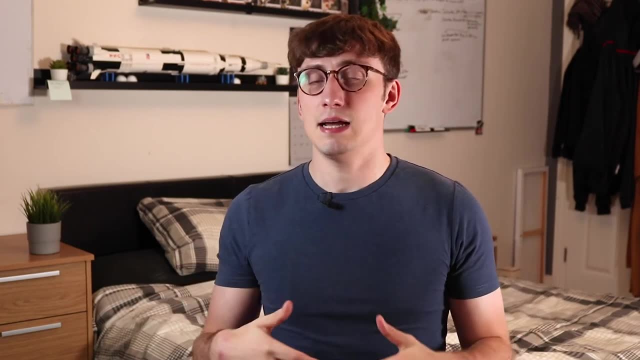 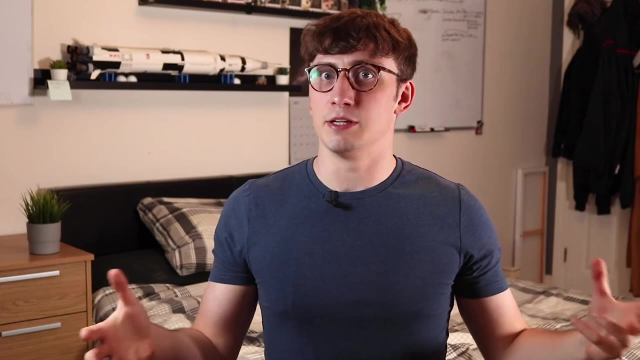 come to be, Then you're probably in it for the wrong reason. Most of my course mates throughout my degree which I was friendly with had a real passion and a real drive to understand these complicated and quite abstract theories about astrophysics. And even then you know. 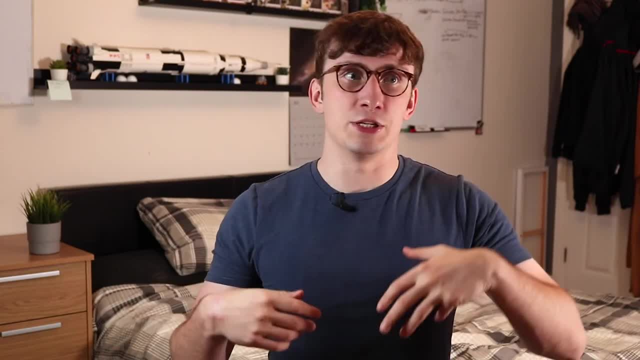 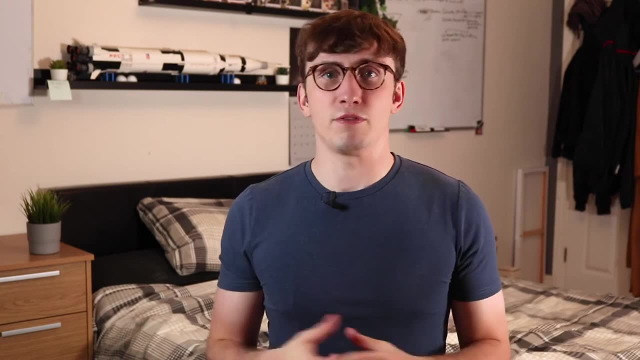 it's easy to lose that motivation when you are facing difficult problems or difficult maths. So that sort of underlying passion is really important to keep that drive throughout the whole degree. Second is to accept ignorance. It's easy to go into an astrophysics degree. 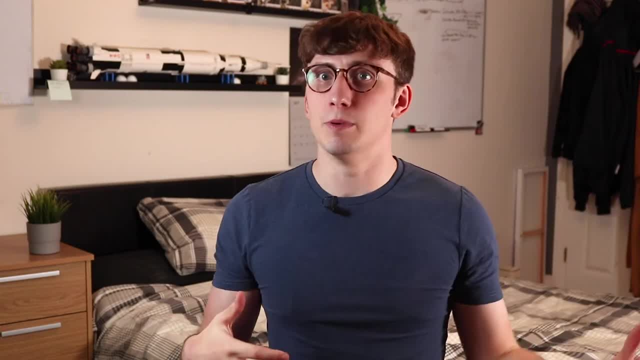 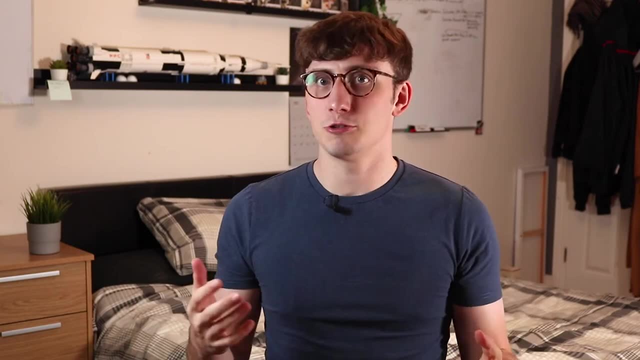 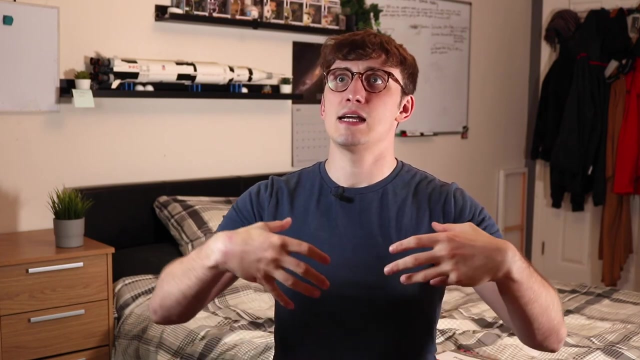 having watched documentaries and YouTube videos and read books on space and astrophysics and think that you've got a pretty good understanding of some of these topics, and the harsh reality is you probably don't, and that's not a bad thing. The best thing you can do is accept the ignorance and embrace the 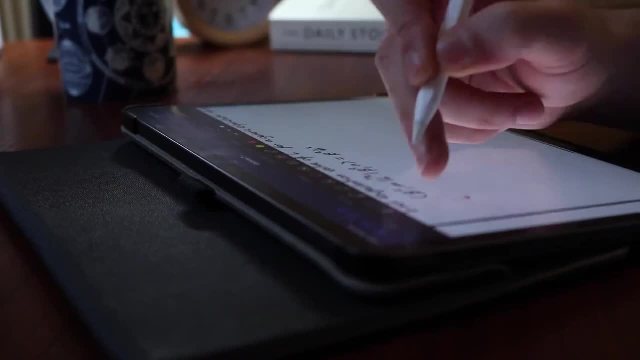 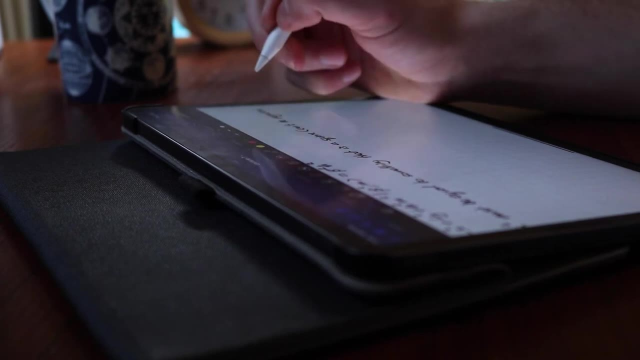 learning process that you're gonna have for university. You're going into university to learn the topics. You shouldn't be expected to know everything already, and so I really recommend then you know, obviously take a massive interest in these topics and watch as many documentaries and YouTube videos. 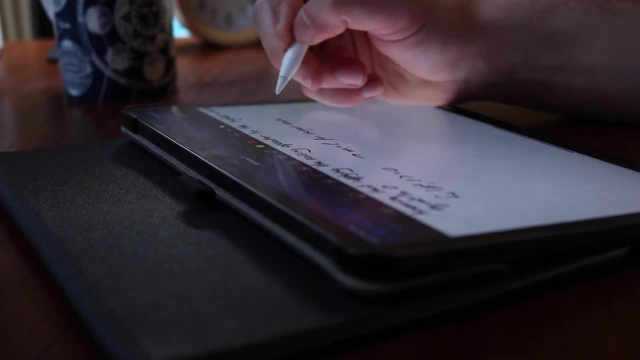 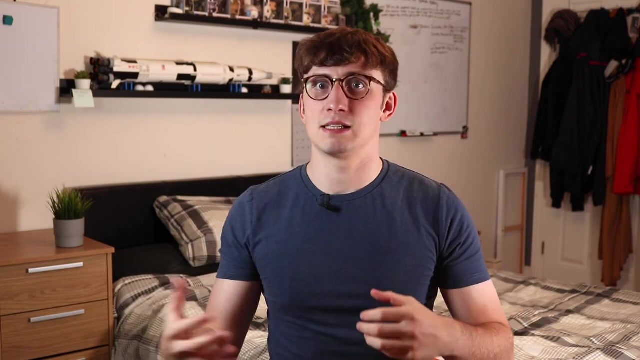 and read as many books as you can on these topics. You know, I had that passion that I talked about in the previous point but I accepted the fact that I'm not gonna know everything about the, the content and the courses that I'm gonna do and that sort of built up a little bit of an excitement for each of. 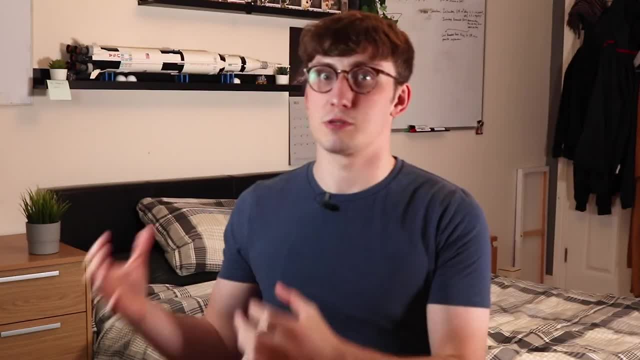 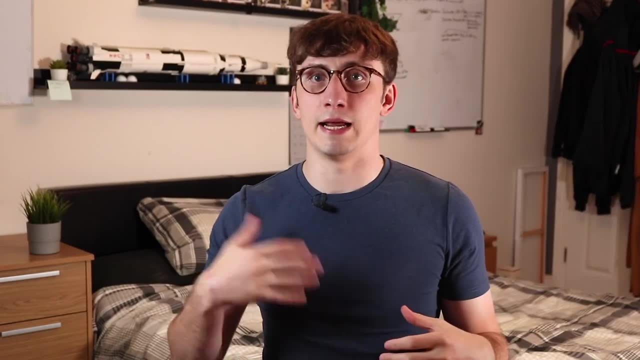 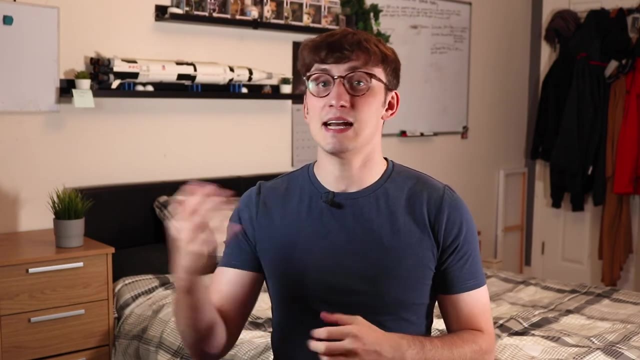 the courses You know. before starting I knew pretty much nothing about cosmology or galactic evolution past the real basics that you've learned through a YouTube video or through an introductory book. but studying those modules actually really sort of built up a drive and a passion that I didn't have before starting. so by 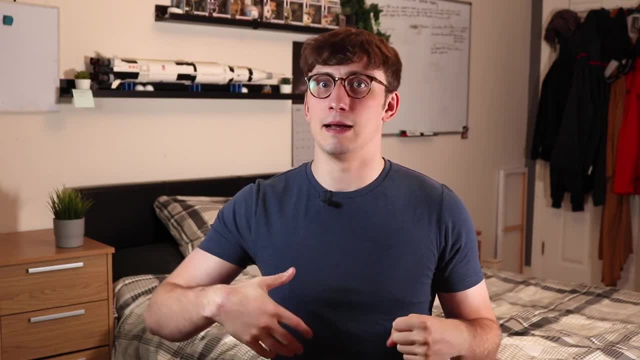 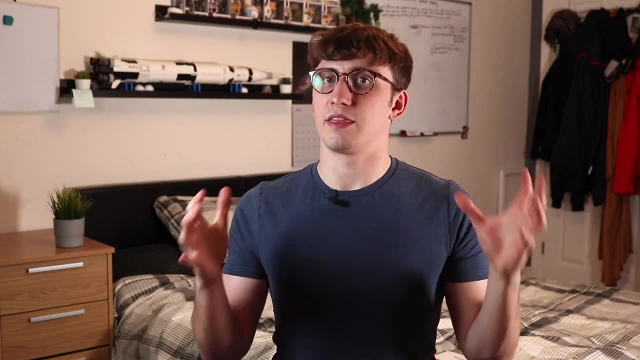 learning. as you go throughout the degree, you're gonna sort of build up the drive and the passion that you have for the subject even more than you did before you started. The final mindset that I think every physics student should have is curiosity, One of the hallmarks of a 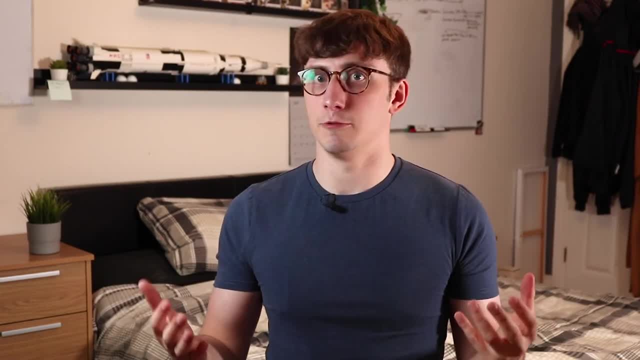 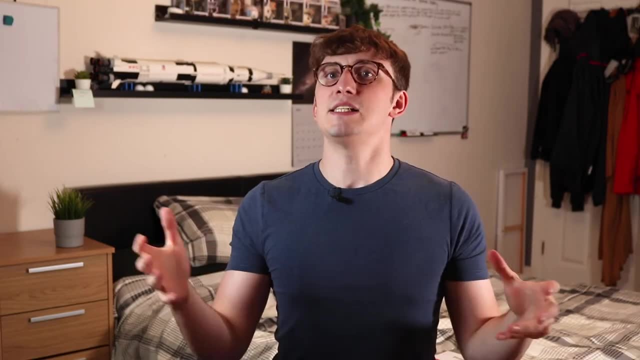 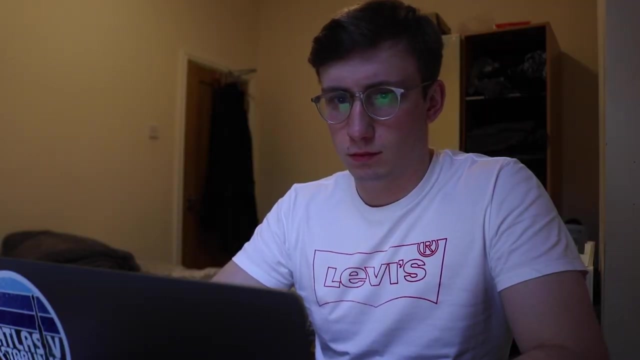 great physicist and scientist more generally, is curiosity and the ability to question and test the facts that we accept as truth. It's easy to think that the content that you're gonna study at university is this well-established science and absolute, concrete facts, and for the most part, it is You know. 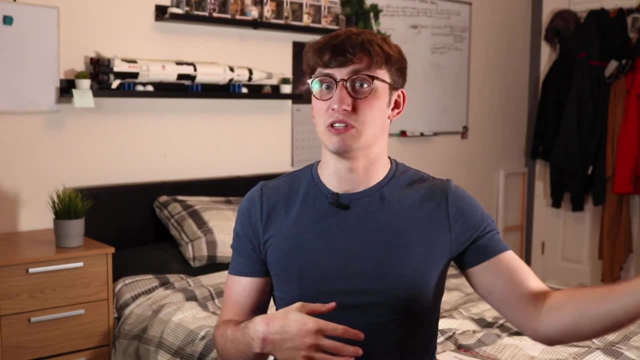 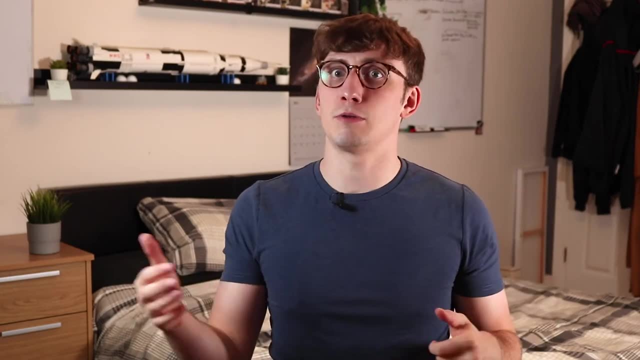 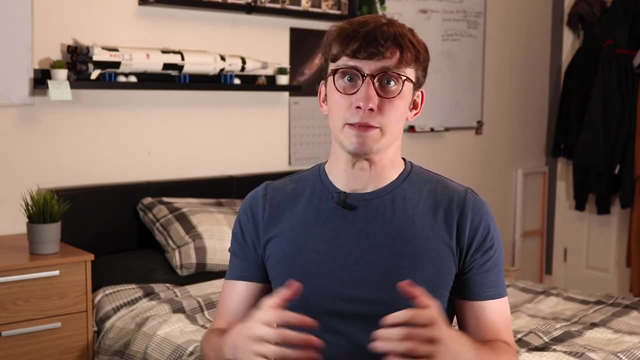 thermodynamics hasn't really changed in decades or even centuries. Mechanics haven't really changed in centuries. but as you move throughout the degree, you get to more and more cutting-edge and revolutionary science. and that stuff is not well established by any means. In fact you know every. 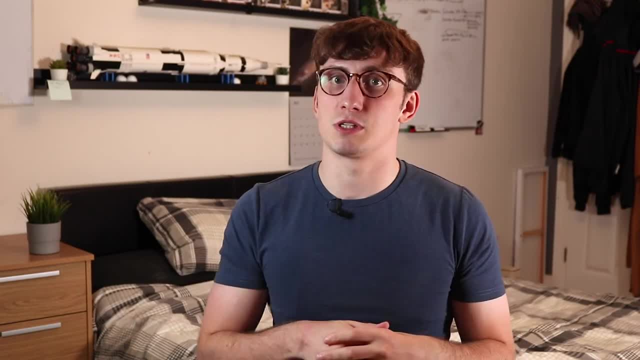 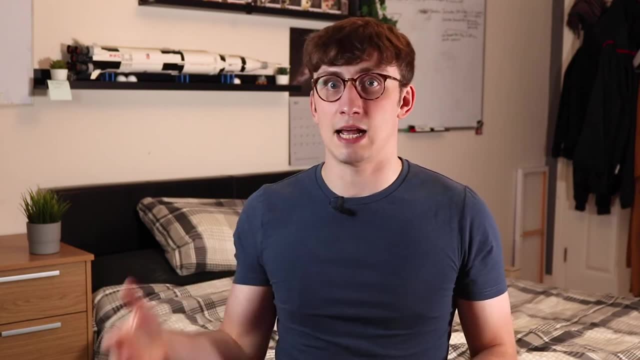 three or four years. they probably have to change little parts of the course to update it with the new science that's coming out. So the theories that we are learning about galactic evolution or stellar evolution might be completely wrong, But I think that's a good thing. 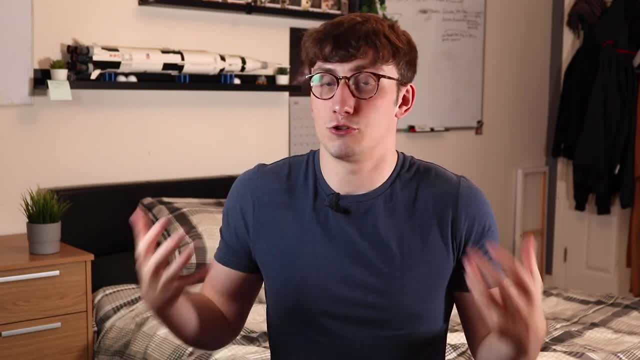 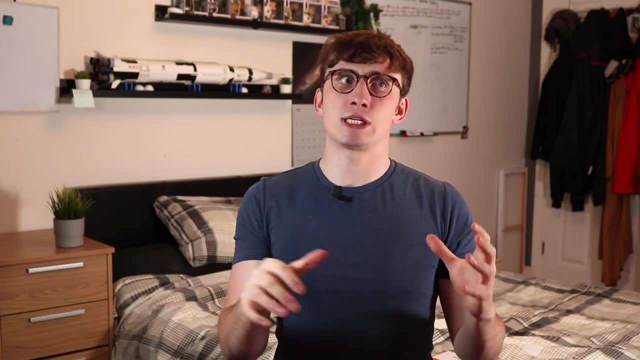 I think that's a good thing. I think that's a good thing. You know they are what we think of as true right now and as more data and more evidence comes to light, we might change those theories. So having that curiosity to question whether the theories of stellar evolution that we're taught is 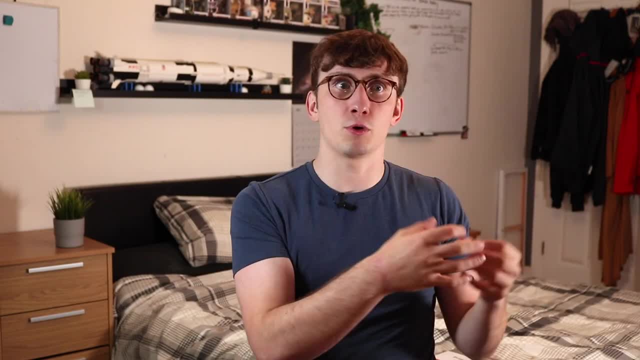 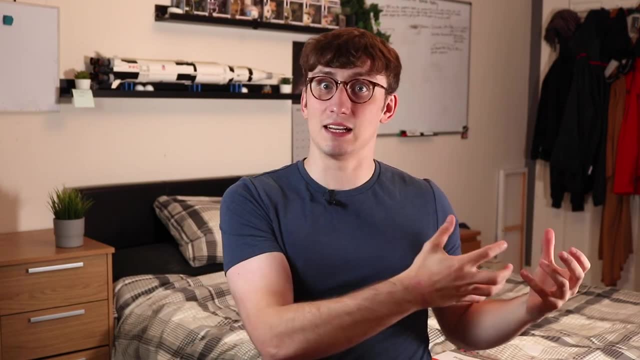 true or whether there's a discrepancy between what we're taught and observational evidence. you know, that is a really important mindset and in fact it's probably a more important skill than anything. So, if you're a physics student, who you know has aspirations of becoming a researcher, 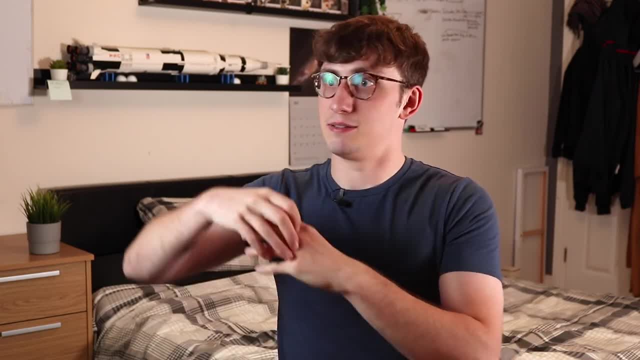 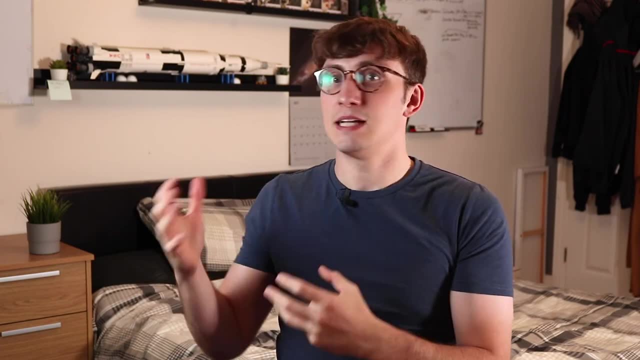 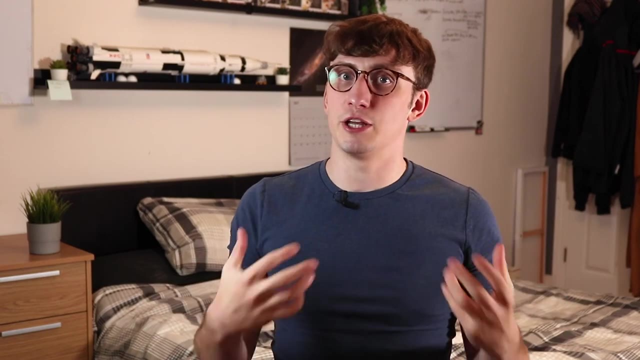 having that curiosity is absolutely vital to question these theories that you know may only be accepted as true because everybody accepts them as true and it's just the norm, And it only takes one person to disprove that theory to birth a completely new field of science. So I really think that curiosity.